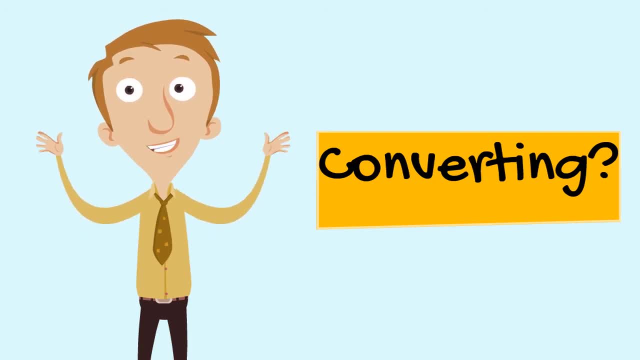 In any other situation, Pause the video and write down an answer. Well, to convert means to change. You might have heard somebody who is converting their garage into a room, Or maybe they're converting the attic into another bedroom. In maths, converting means changing measurements from one unit to another. 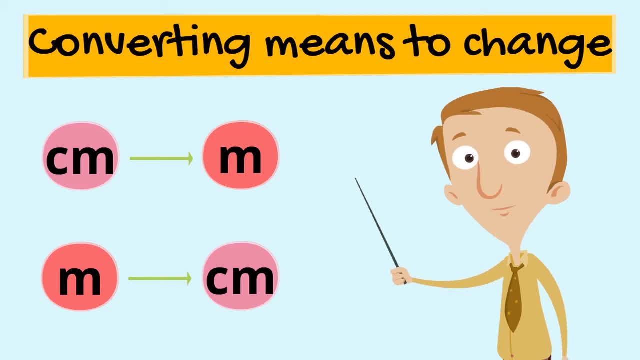 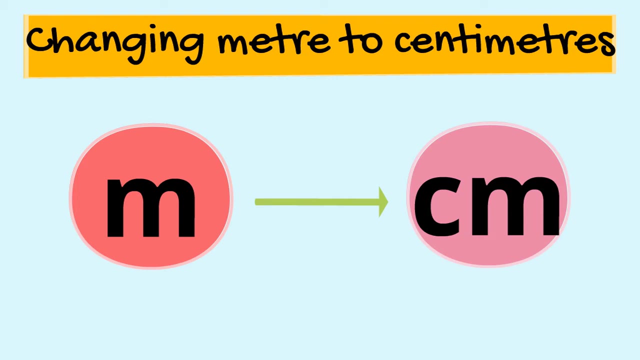 Today we're going to be looking at how to convert centimetres into metres and how to convert metres back into centimetres. Let's start off by changing metres into centimetres. Have a look at the examples below. All of these are correct. 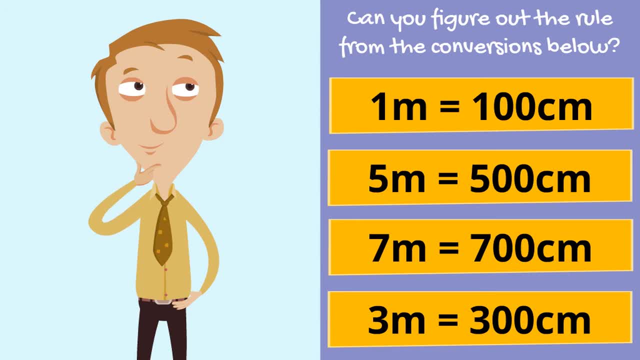 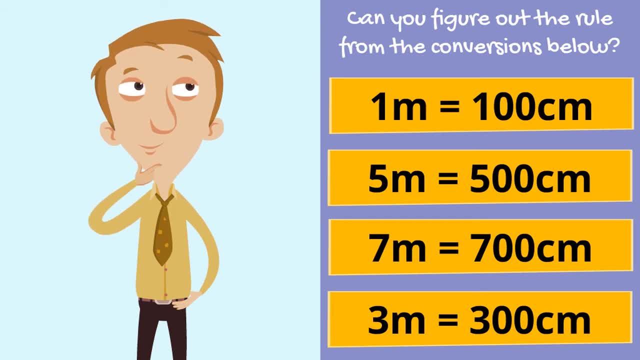 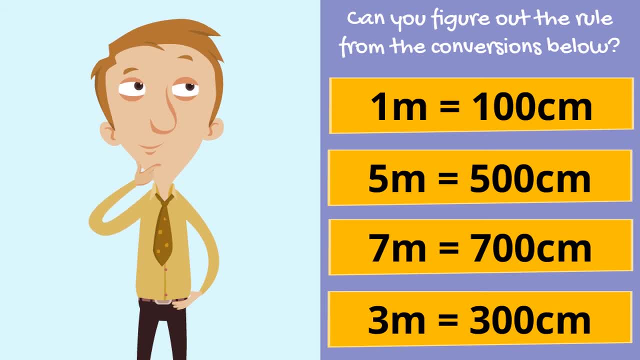 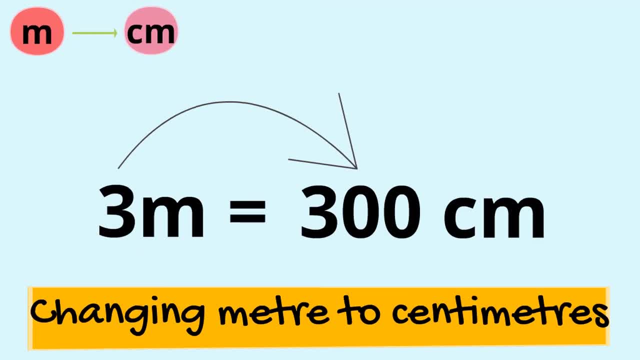 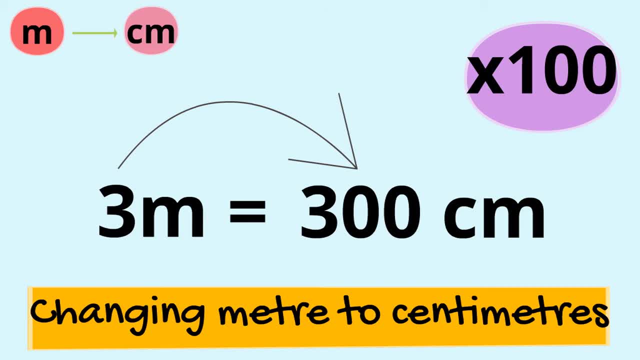 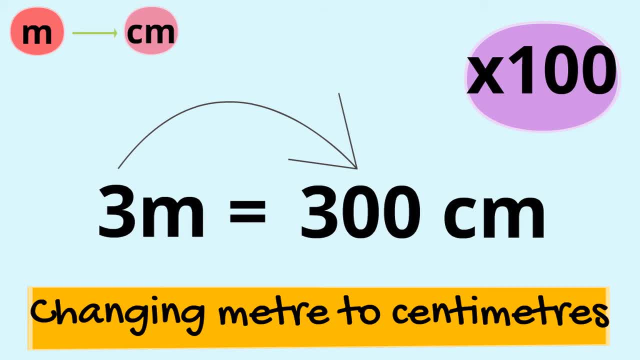 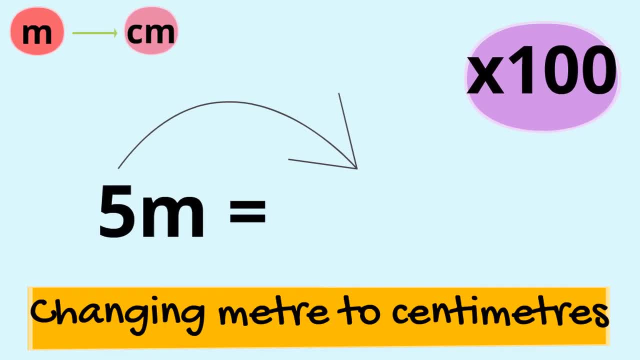 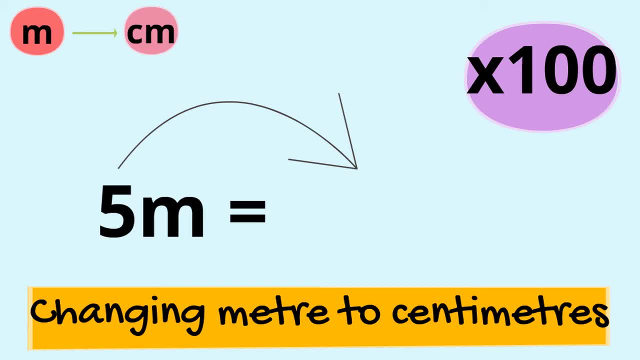 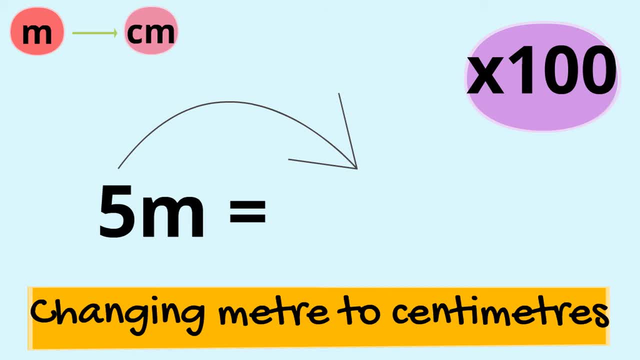 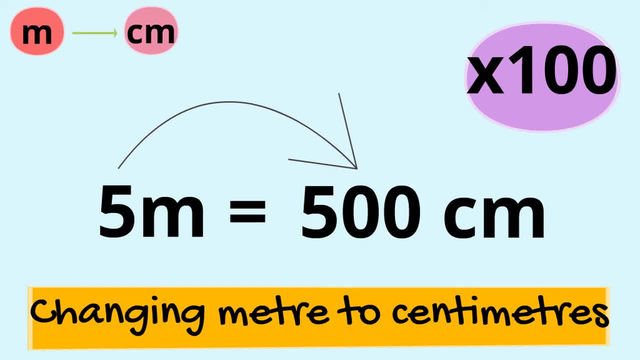 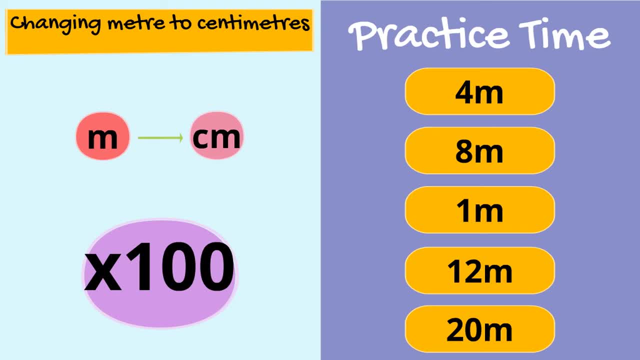 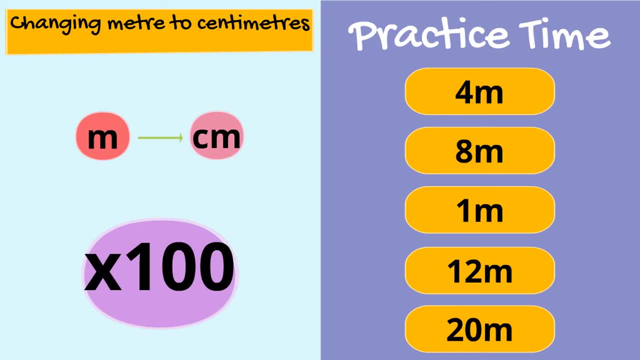 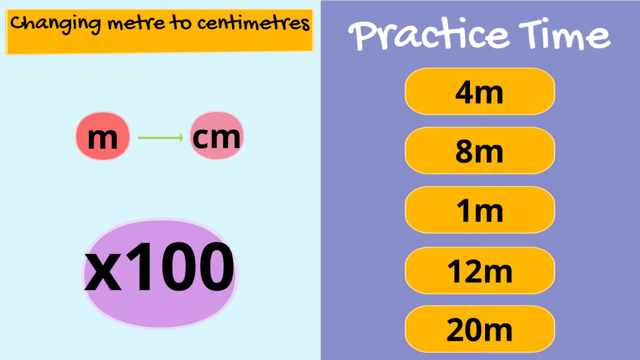 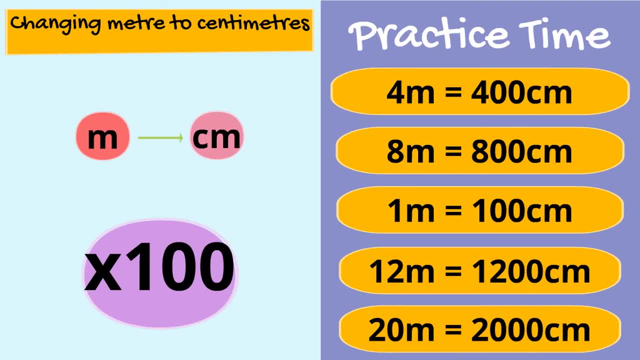 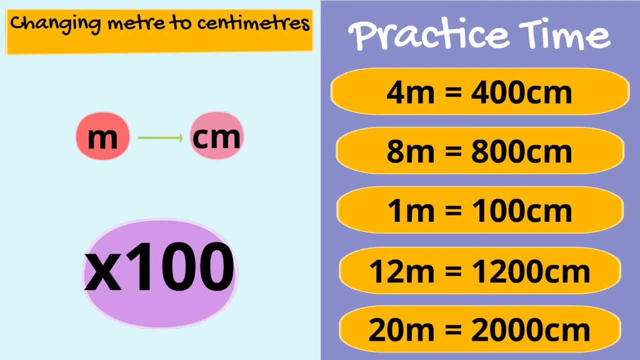 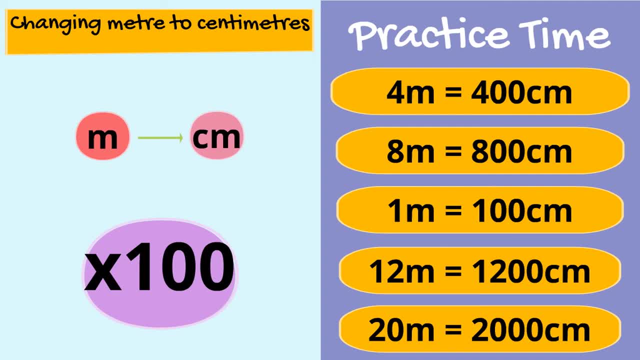 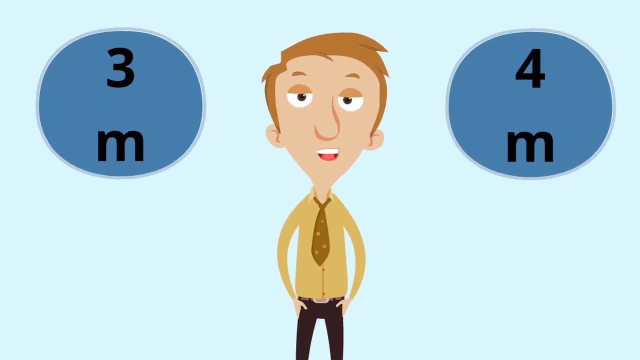 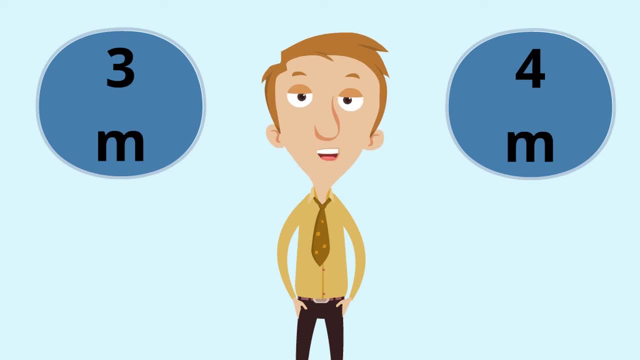 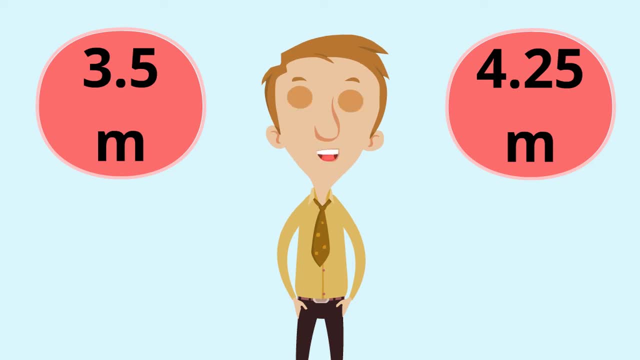 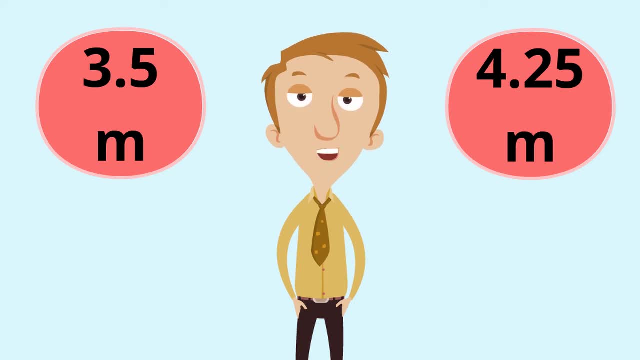 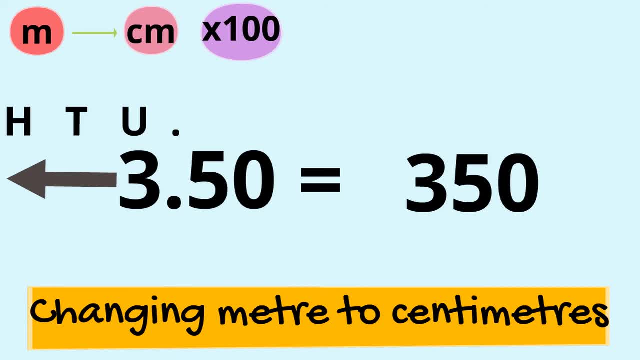 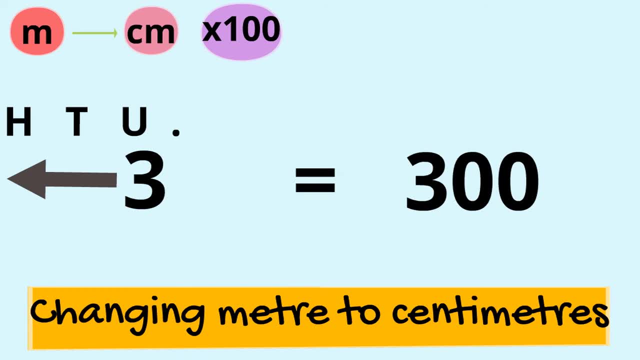 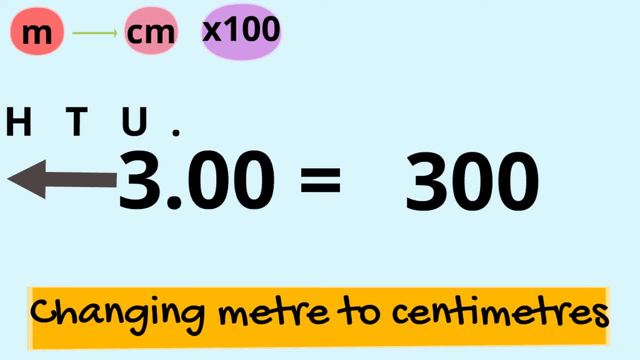 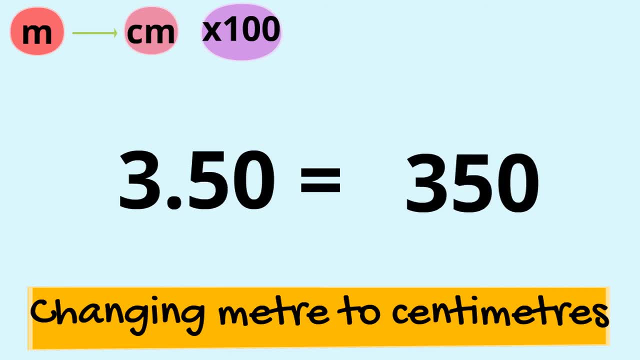 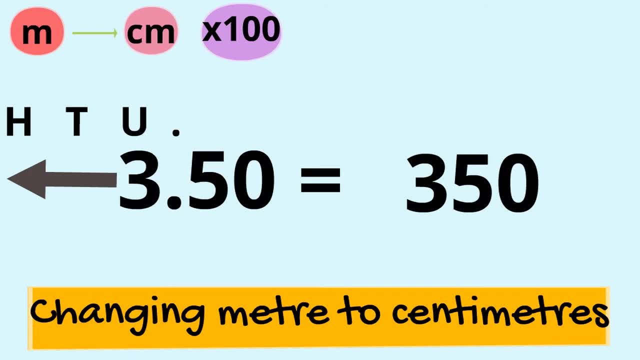 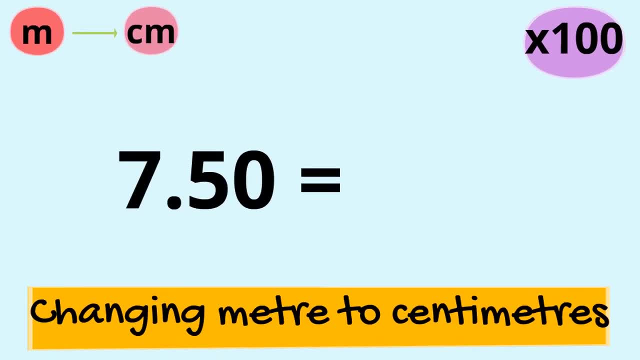 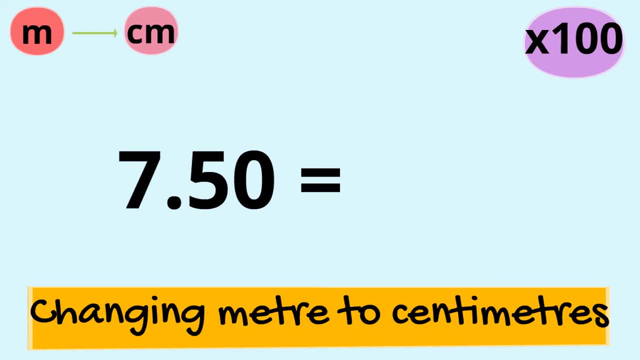 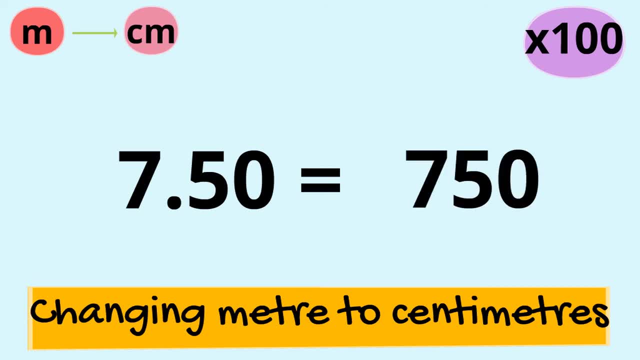 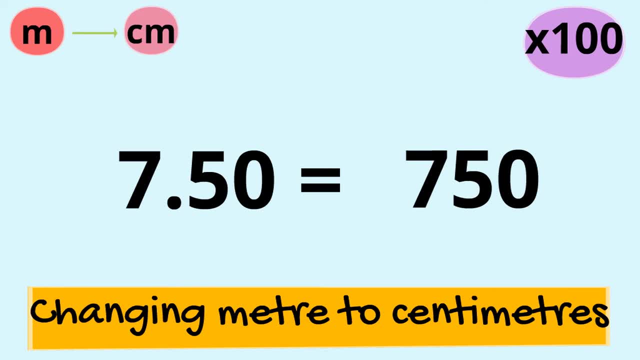 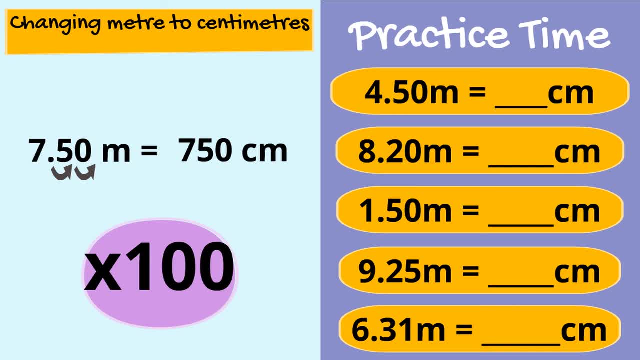 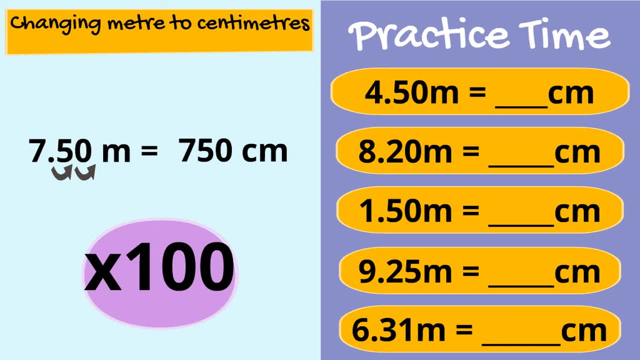 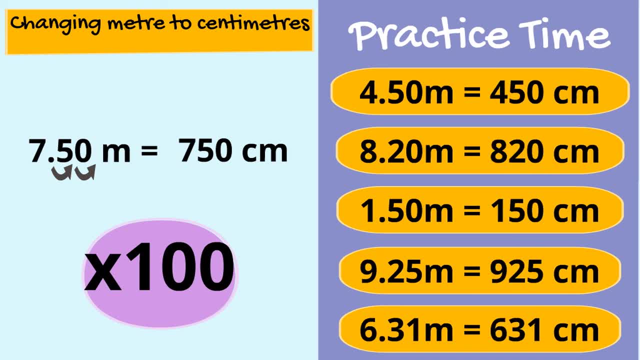 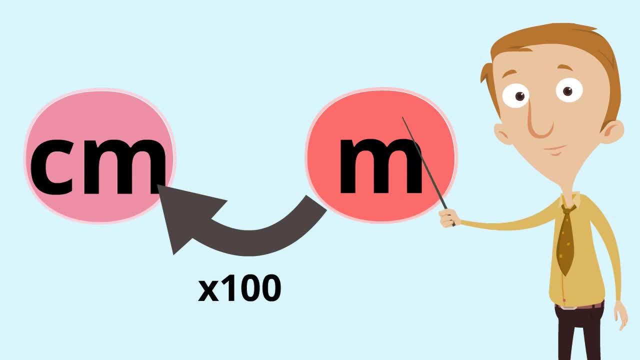 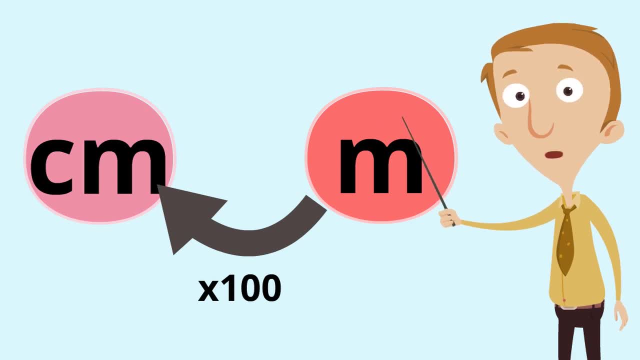 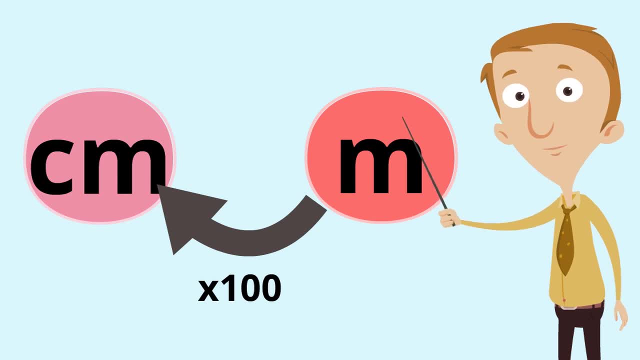 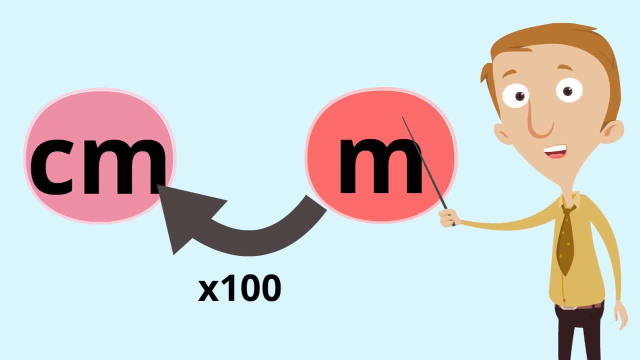 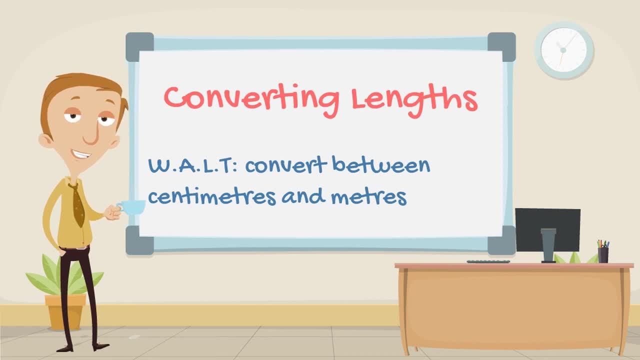